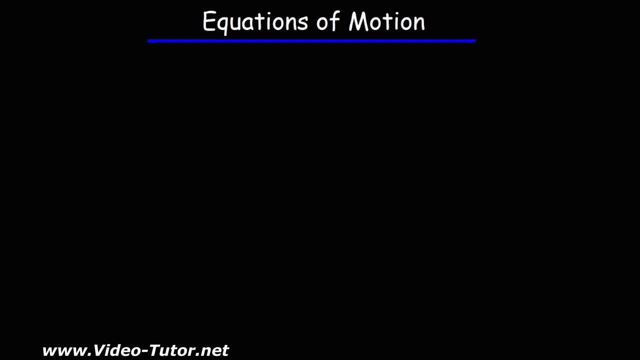 So let's talk about equations of motion. So the first thing you need to identify when dealing with problems associated with equations of motion is if the object that's moving, if it's moving at constant speed or with constant acceleration. So let's start with constant speed. 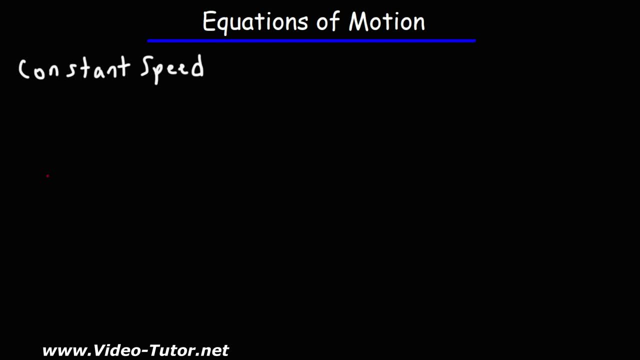 If an object is moving with constant speed, this equation becomes important. d is equal to vt. Now d can be used as distance or displacement, So you can think of distance as equal to rate multiplied by the time. or distance is equal to speed multiplied by the time- Same thing. 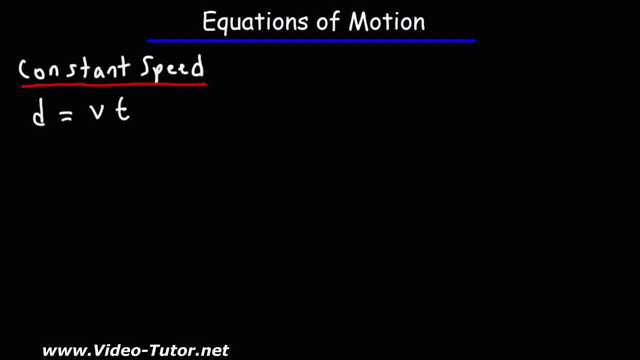 Or you can think of displacement as equal to velocity multiplied by time, And, of course, you can rearrange this equation If you're calculating the speed, which is the same as v. speed is equal to distance divided by time. Velocity, on the other hand, velocity is equal to the displacement over time. 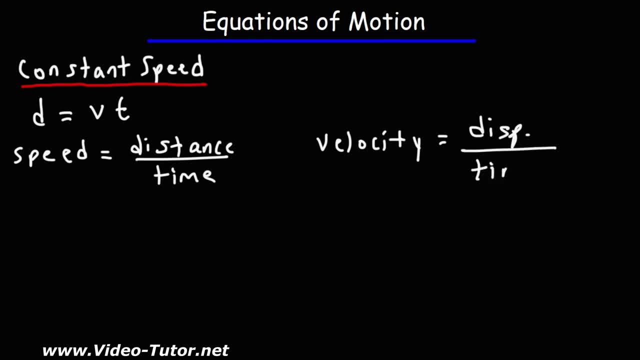 Now remember, Velocity is a vector, Speed is not. Velocity has both magnitude and direction. Speed only has magnitude. Speed is always positive. However, velocity can be positive or negative. So speed is the absolute value of velocity. Now, if you're wondering what the difference between distance and displacement is, distance is a scalar quantity, like speed. 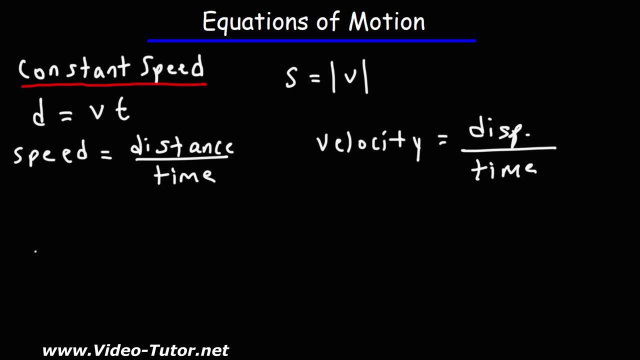 Displacement is a vector quantity, like velocity. So let's say, if a person travels 8 meters east and 3 meters west, the total distance that this person travels is 11 meters. Distance is always positive. Now the displacement, however, is different. 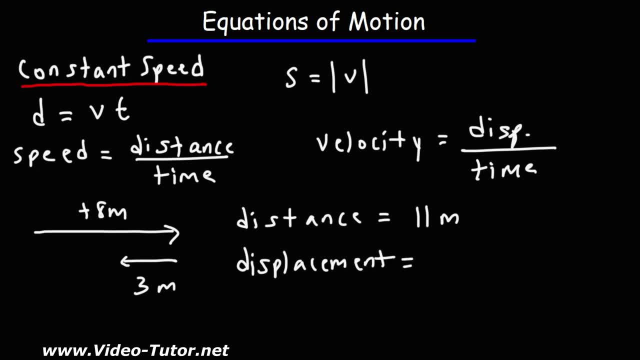 During the first part of the trip the displacement is positive because he's traveling. He's traveling east towards the positive x-axis. But during the second part he's traveling west and that's negative. So to calculate the displacement you would add these two. 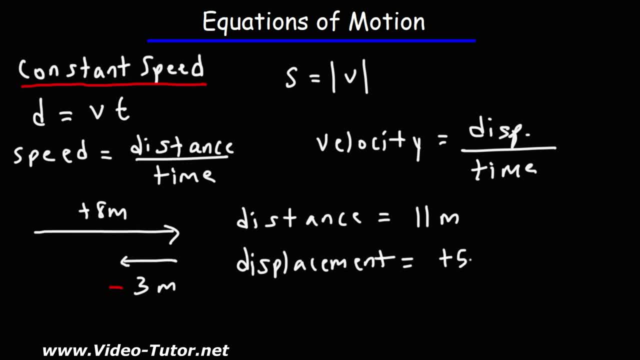 Positive 8 plus negative 3. So it's positive 5 meters. If you look at the difference between the initial position and the final position, you would also get 5.. So that's displacement. Displacement is the change in position. 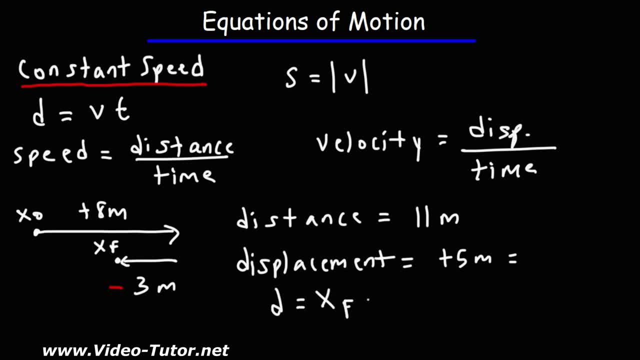 So you can calculate that along the x-axis The final position minus initial position, So that's horizontal displacement. Or you can calculate the vertical displacement, dy, which is also the final position minus the initial position. Now going back to velocity. 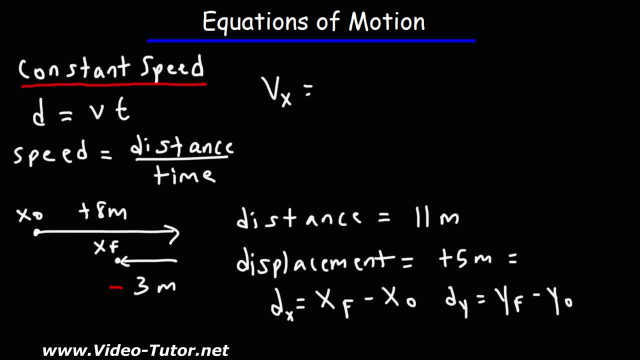 If you want to calculate the velocity in the x-axis, you would need to calculate the velocity in the x-axis. You need to take the horizontal displacement, which is the final position, minus the initial position, and then divide it by the time. If you want to calculate the vertical velocity in the y-direction, you need to take the final position minus the initial position in the y-direction, divided by t. 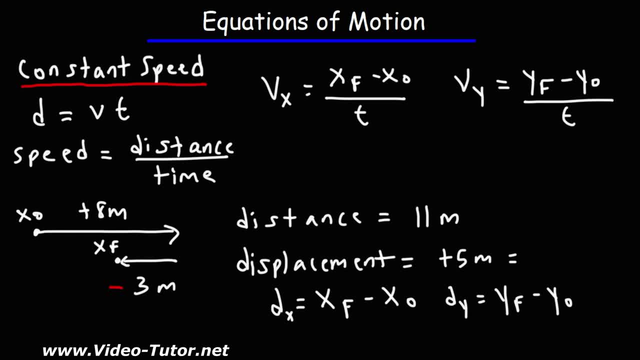 So pay attention to the direction in which you're calculating velocity. Is it in the x-direction or in the y-direction? It's in the y-direction. Now let's move on to the formulas you need to know when dealing with constant acceleration. 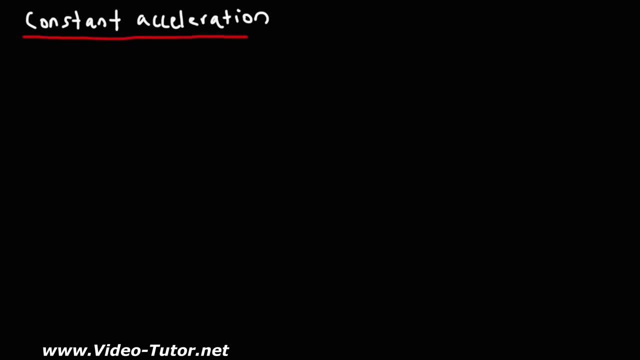 Keep in mind: velocity is the rate at which displacement is changing. Acceleration is the rate at which velocity is changing. So, as we saw, velocity was displacement over time. Acceleration is the change in velocity over time. So acceleration is delta v over delta t. 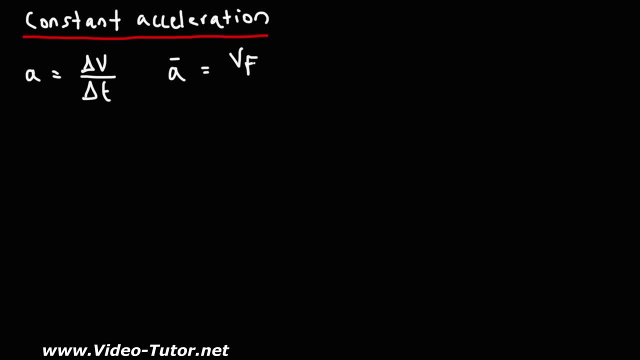 Particularly. this is average acceleration. So it's v final minus v initial divided by t. Now if you were to rearrange this equation, if you multiplied a by t and then added v initial, you would get v final. You would get: v final is equal to v initial plus a t. 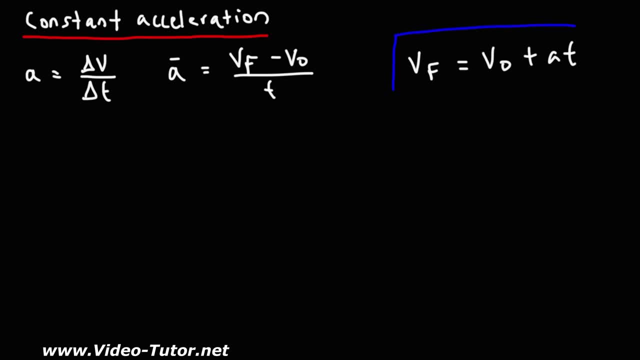 By the way, for those of you who want example problems on how to use these formulas, check out the links in the description section below. I'm going to post some videos, like on kinematics, projectile motion, free fall problems, and in order to solve these problems, you need to use these formulas. 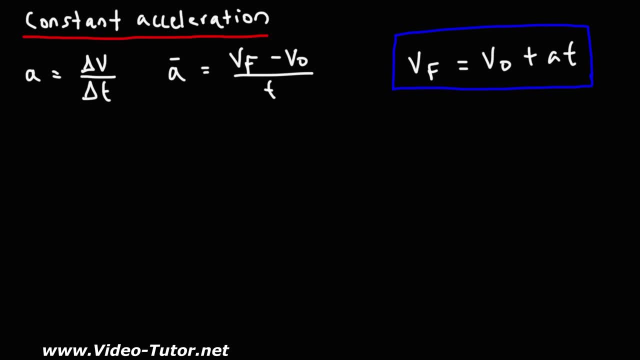 So it'll give you the practice that you need. The next formula you want to be familiar with is this one: v final squared is equal to v initial squared plus 2 a, d. Also, pay attention to units. Velocity is typically in units of meters per second, feet per second miles per hour, so forth. 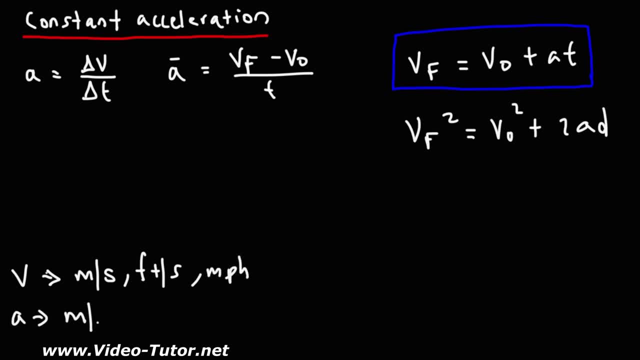 Acceleration is like meters per second squared, feet per second squared and things like that. It could be kilometers per square hour. It's unit left over time squared. Now recall that for constant velocity we had this equation d is equal to vt. 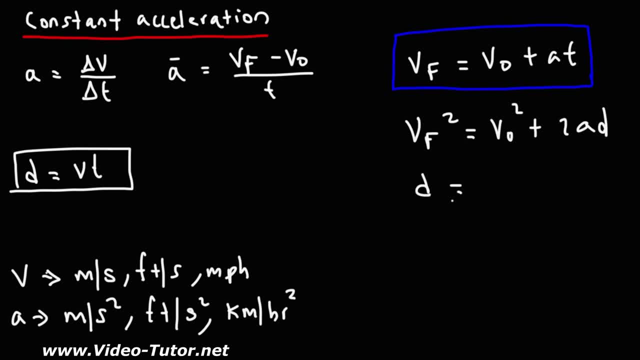 For constant acceleration. it's very similar but because we have acceleration, the velocity is changing, so you need to use the average velocity. Whenever you want to find the average of two numbers, you need to add up the two numbers and divide by 2.. 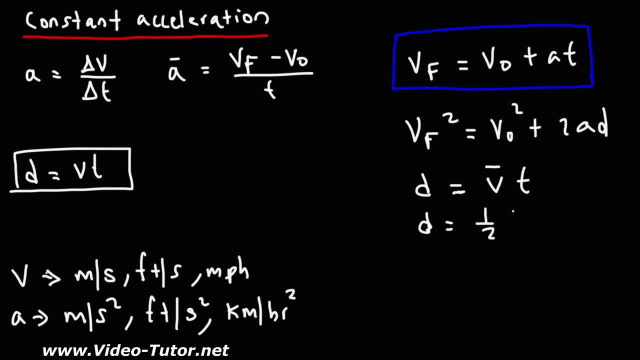 So dividing by 2 is the same as multiplying by a half, and then we're going to add the initial and final velocity values in this time interval. So that's the next equation. you need to calculate displacement: It's the initial velocity plus the final velocity divided by 2, multiplied by t. 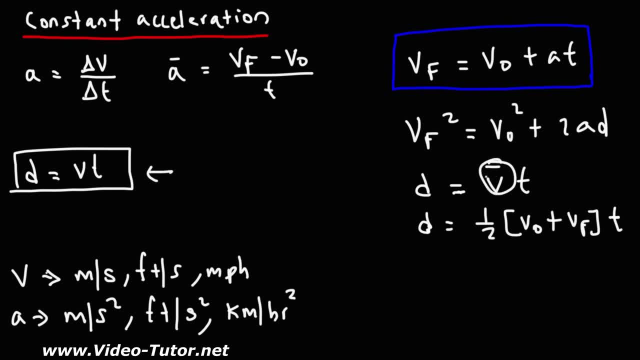 But it comes from this equation. It's just that we're using average velocity instead. Now, displacement is also equal to v, initial t plus 1, half at squared. Now I've seen different variations of this formula because, mind you, you can replace displacement. 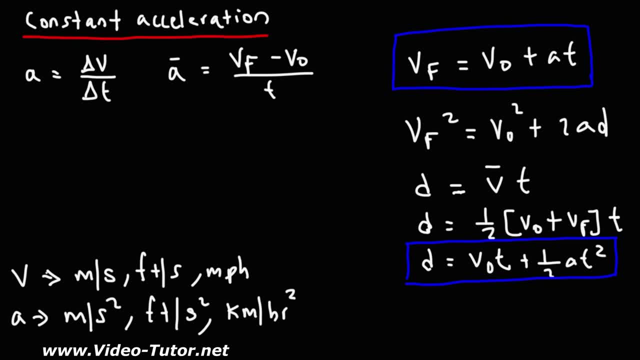 with final position minus initial position in the x or y direction. If you replace it with the x direction and solve for final position, you get this equation: Final position is equal to initial position plus the v, initial t plus 1 half at squared. 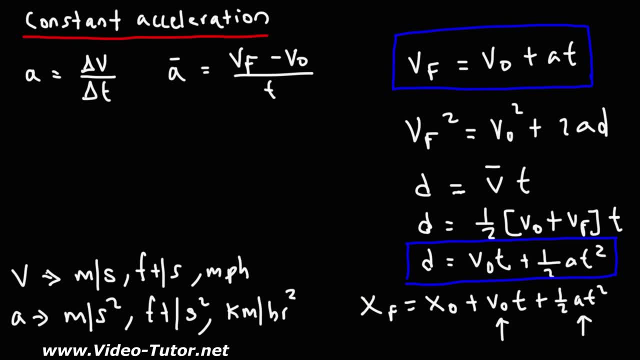 In this case, the initial velocity and the acceleration are all in the x direction. Now you can apply the same formula in the y direction and it's going to look like this: In this case, v initial is in the y direction.